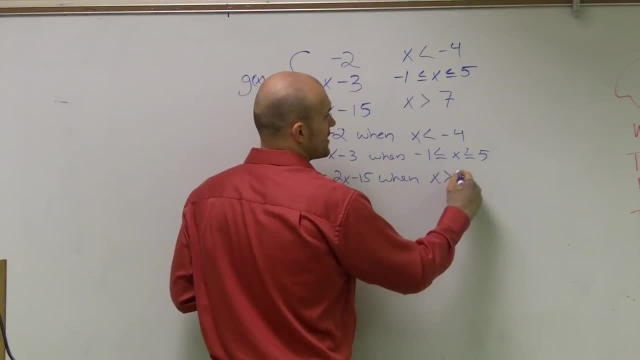 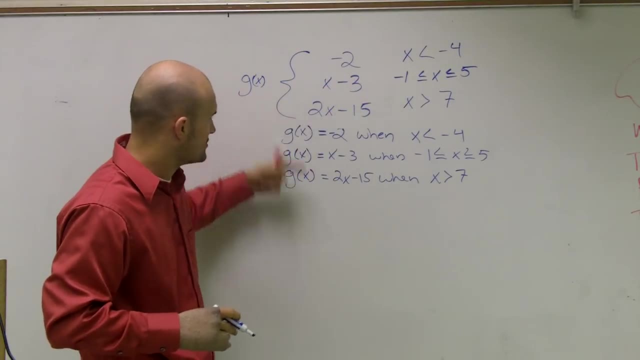 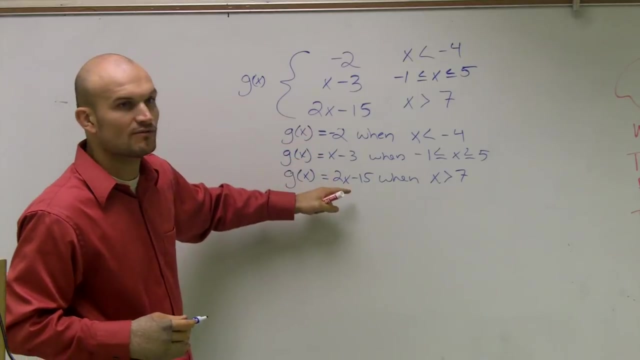 only when x is greater than 7.. Now, these aren't g of x, because actually g of x is all of them combined, But I had to use a function, so I used g of x again, But notice, g of x is the function of all three of these combined. These are all individual functions that we need to graph. 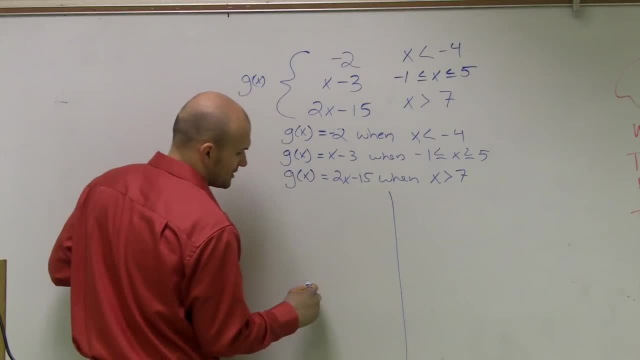 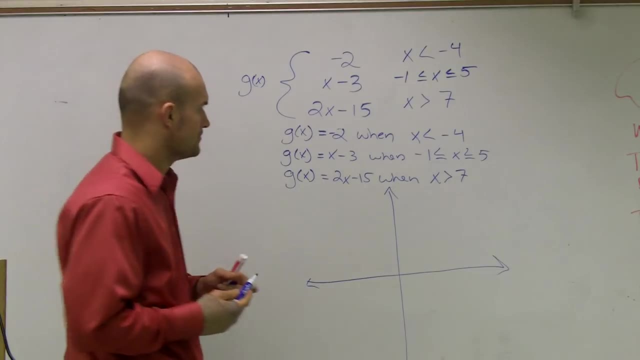 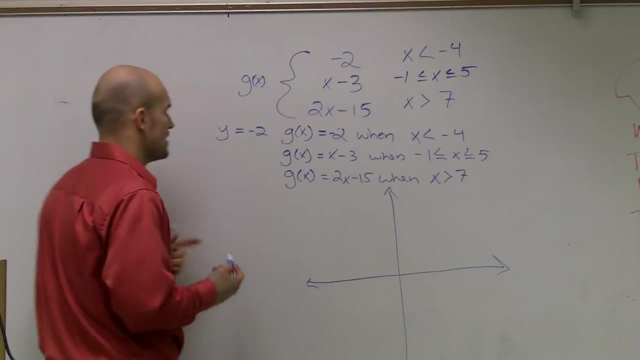 So what I'm going to do is I'm going to have to graph each one of these separately, according to their constraints. So if I need to graph negative 2, remember, think of that as like a y and an x. y equals negative 2.. If you're going to graph that on an x and y plane, you're 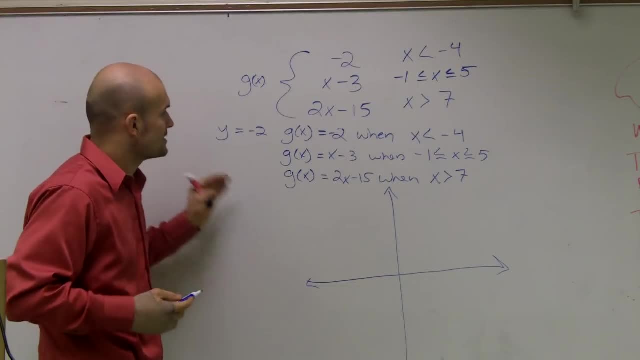 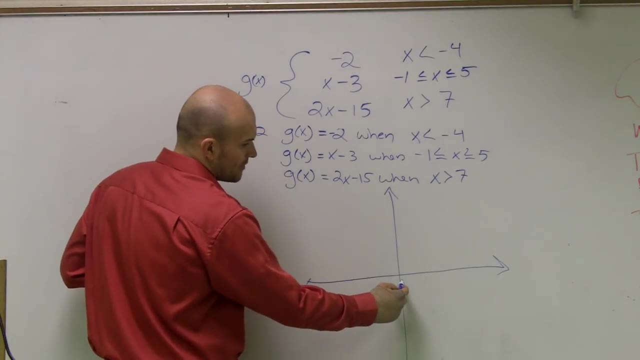 not going to write whatever you take. So I'm going to graph this on an x and y plane. And now what I'm going to do is I'm going to take the two x's plus this left over here. So I'm going to get the first two x's that we picked, and that one's going to be. 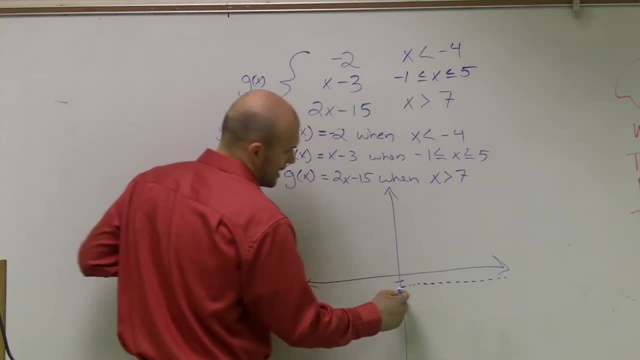 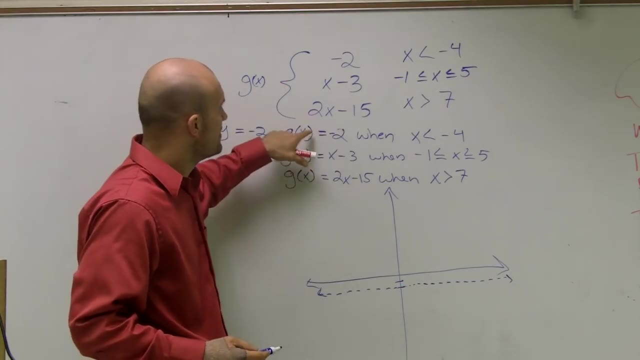 negative 2.. So we're going to show you an example of this. So again, we've got an x. So specifically, we are going to get an x that's going to be equal to that, And then we're just going to compute the equation for that x. 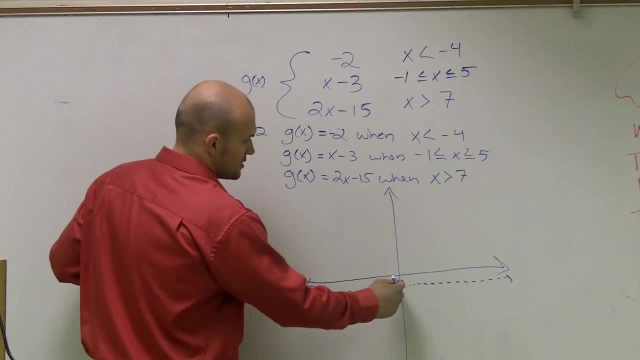 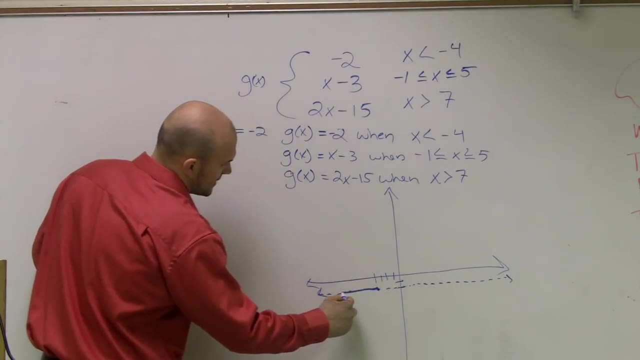 So look at these. OK n than negative 4.. So I go to negative 4.. 1,, 2,, 3,, 4.. So that means this graph is only true from this point on. Then I need to determine, since it's an open circle. 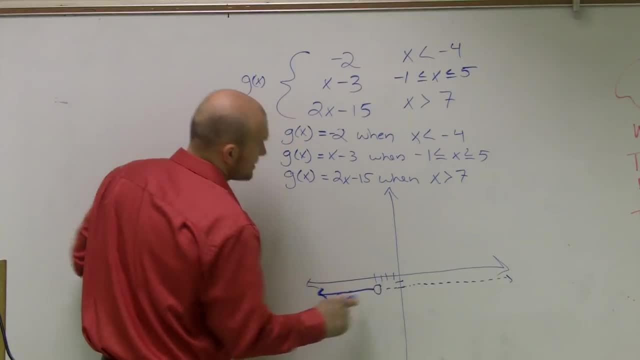 that's going to be an open dot Right, Because it does not include the point negative 4.. So the rest of this, even though I wrote it down a line, it really has no effect. It's not part of my graph or not part of my function. 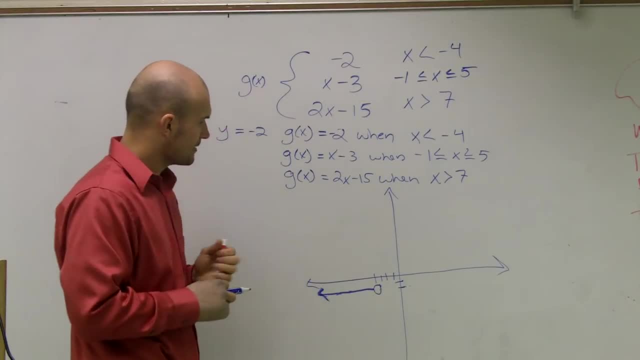 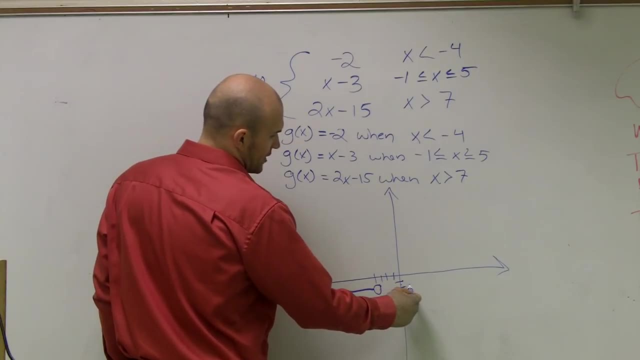 GeoVax. my piecewise graph. The next one: x minus 3.. I need to graph that So that crosses at a y-intercept of negative 3 and has a slope of 1 over 1.. So that looks something like that. 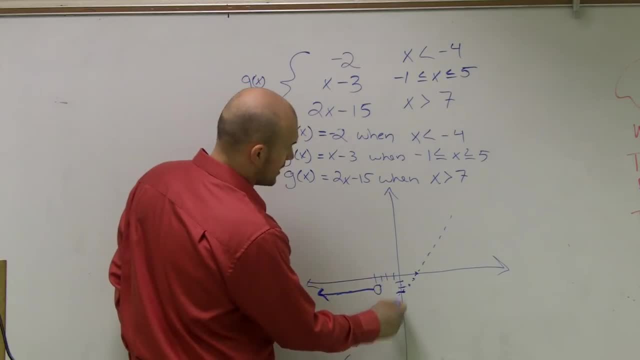 Now that graph is only true between negative 1.. And since it's now less than or equal to, that's going to be a solid dot: less than or equal to 1,, 2,, 3,, 4, 5..